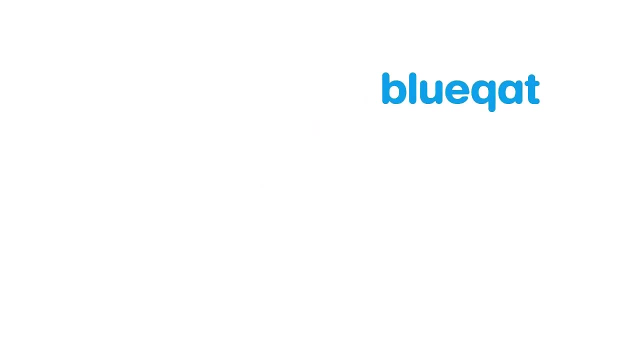 In this tutorial video, we will be learning on Deutsch-Jozsa Algorithm. Deutsch-Jozsa Algorithm Overview. It describes the Deutsch-Jozsa Algorithm, which is a generalization of the Deutsch algorithm. The Deutsch-Jozsa algorithm assumes that this f. 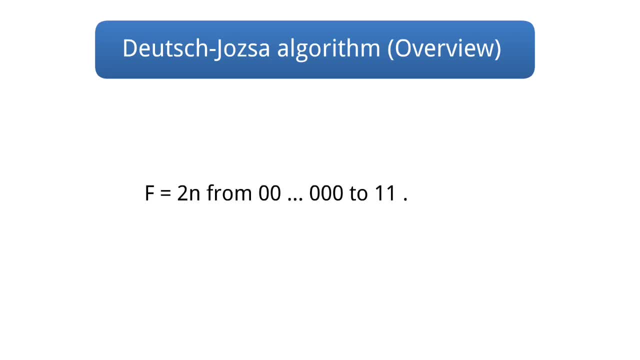 input is 2 to the power of n, from 0, 0 to 1, 1, and one of the following conditions is true. first, f of x is the same for all inputs. f of x equals 0 for all x, or f of x equals 1 for all x. 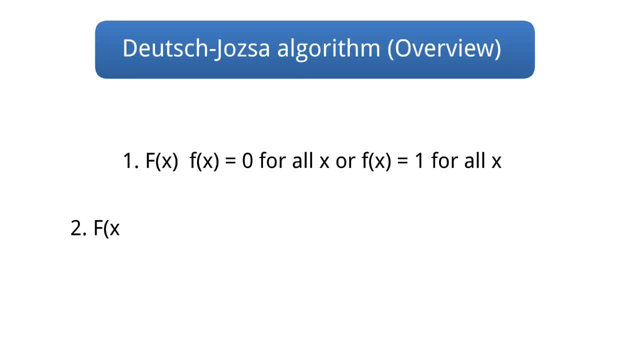 second, f of x is different in half of the inputs. 2 to the power. n minus 1, and x is f of x equals 0. the remaining x is f of x equals 1. this algorithm determines whether oracle is 1 or 2 above. 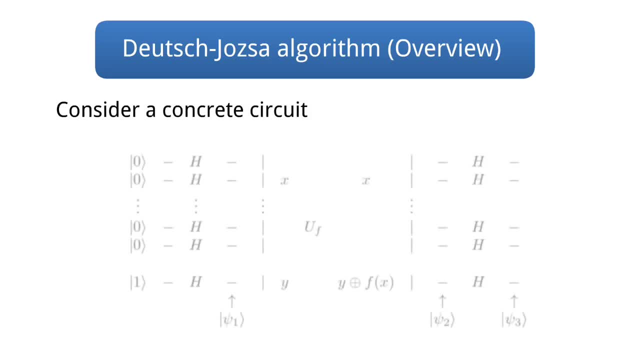 consider a concrete circuit. it is assumed that n zeros are lying on top of each other and that n zeros are lying on top of each other up. let's check each status. looking at the nth bit, we can see that swapping zeros and ones changes the overall sign. next consider psi 2, since f of x is on the nth bit. it will be if you divide the. 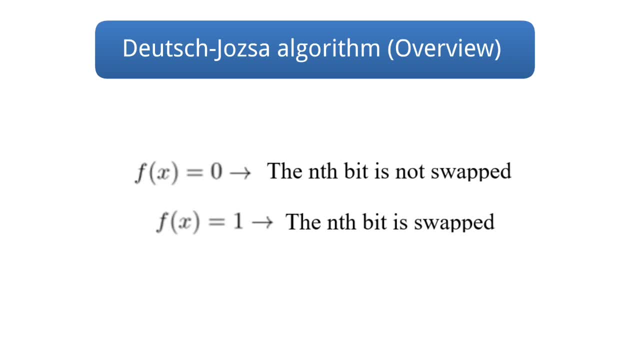 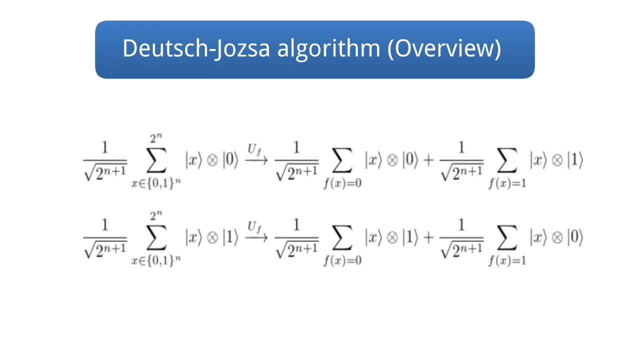 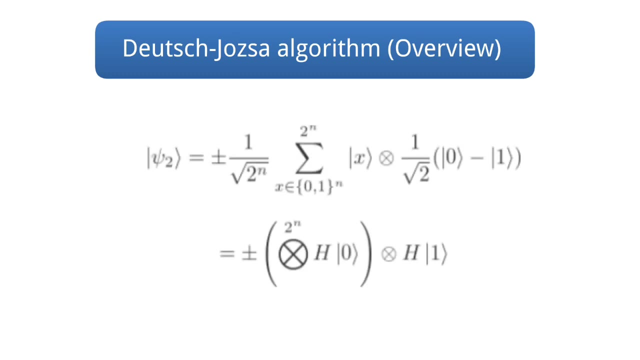 sigma by f of x equals 0 comma 1 for each term. you can see that the bits have changed when f of x equals 1. summary: therefore: when it is 1 either, the sigma of f equals 0 comma 1 disappears. also, when it is 2, sigma remains in both cases. so no further calculation is possible from the above. 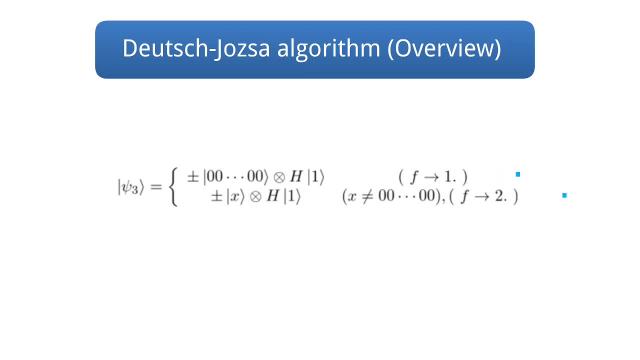 psi 3 is unless the top N bits of site 2r H 0 greater than H 0 greater than the top end bits of site 3, cannot be 0: 0. so you can see that Psi 3 is multiplied as above, since plus, minus is irrelevant to the minus, plus related feedback corresponding to excellence, as the number of integer values, blade is correct, or 같아, and diameter, respectively. 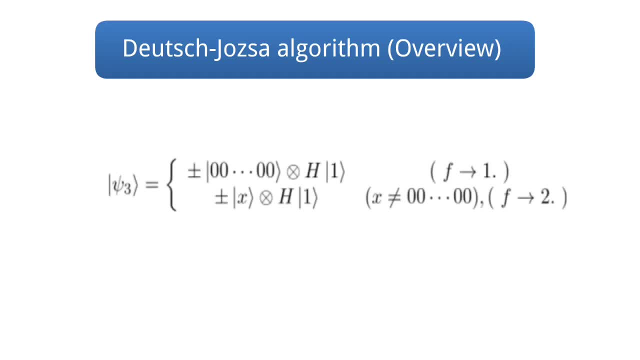 as Bigger than h0, greater than the top end bits of Psi 3 cannot be 0. so you can see that Psi 3 is multiplied, is increased and ever more so. x is the operative and y is multiplied as above. t plus minus is irrelevant to the minimum result to transform to a further algorithm.